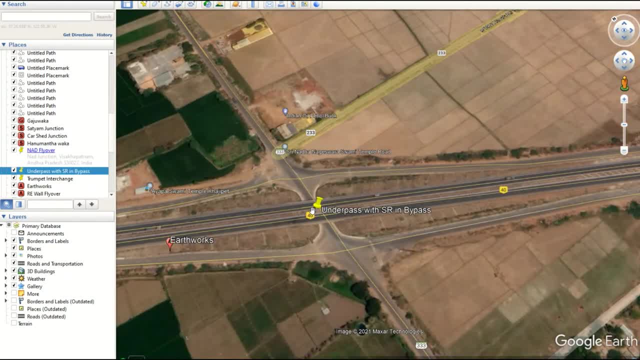 bridge portion in this portion. what type of cross section that we will get it from? the specific code that is nothing but IRC, SP 84, or else SP 73, whatever means, if it is a four lane, it's 84, if it is a six lane, SP 86. so like that you. 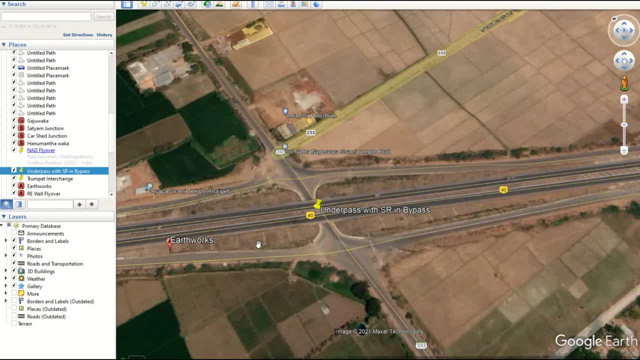 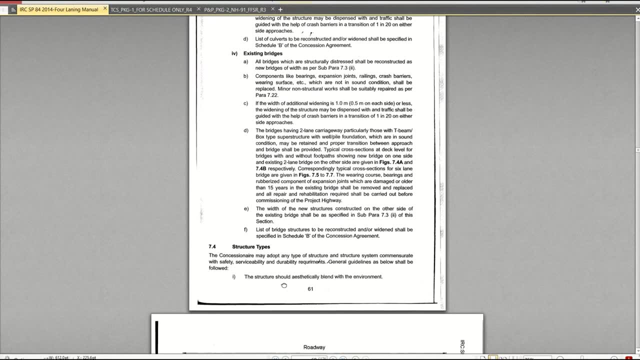 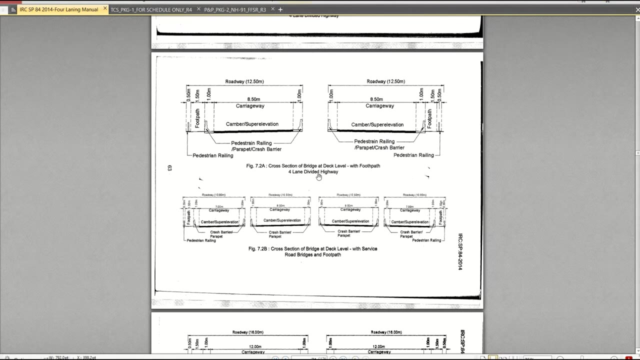 have to refer particular cross section right, I will show that. you can see figure seven point to be like that in IRC: structure types, based on the structure types you have to, you know, see pedestrian trailing. this is for the footpath. okay, at deck level, with service road bridges and footpath. okay, six lane. 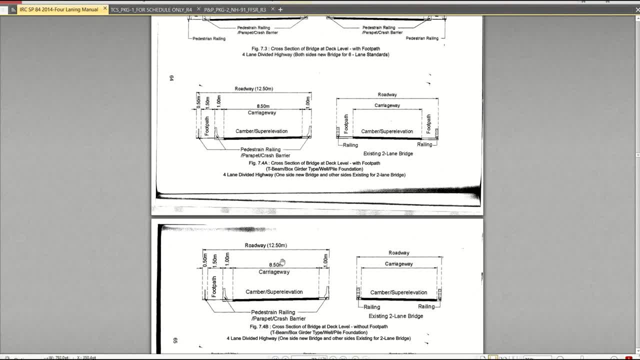 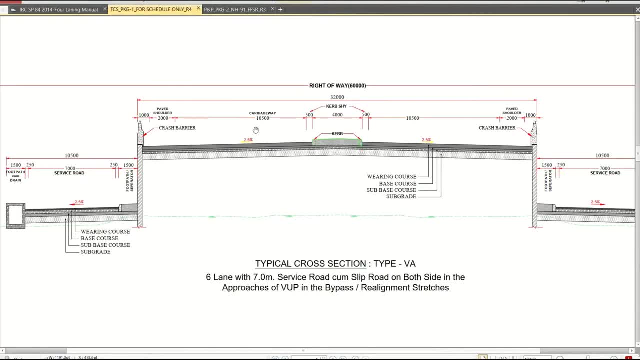 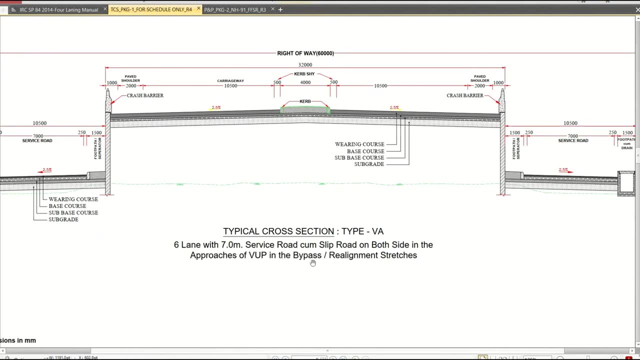 bridge. okay, so, according to the requirement, you have to consult with the structure team and you have to propose a specific cross section and you have to prepare something like this. can you see, this is specially for the V UPS in bypass or the element structures with service road on both sides- you have to prepare a typical slash. 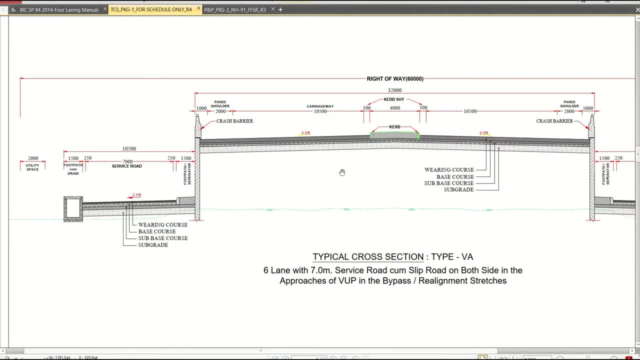 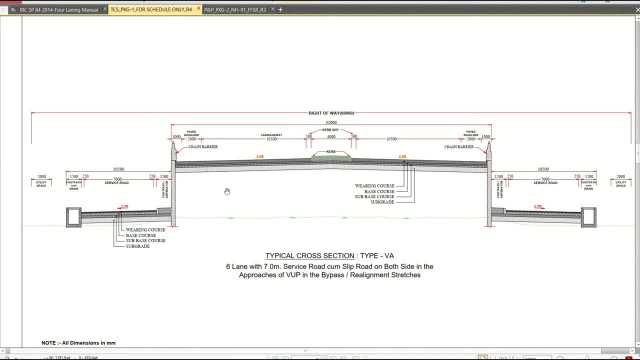 action for submission purpose. but in open roads and civil 3d you have to create a template separately to carry out quantity or whatever, okay, but in MX Road it's not required. you have to prepare a typical cross section and we have to run a line mode with respect to the details provided in the process. 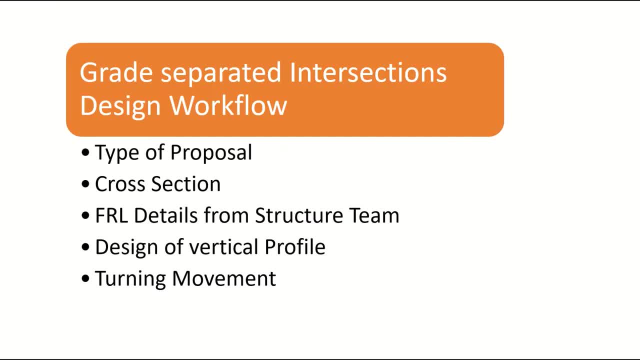 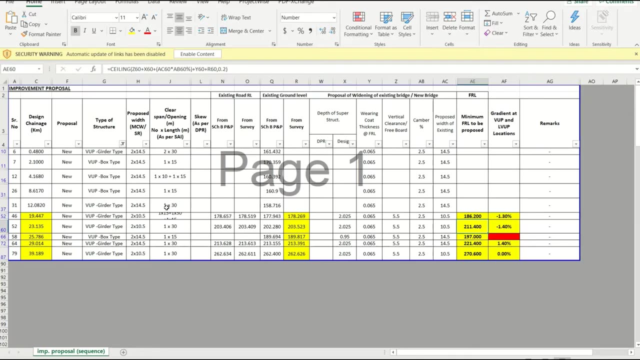 in the typical crash section. okay, so this is the second. next one is frl details. how to get that frl details? you know getting frl details from the structure team, but you must be aware about the process. let me show the excel sheet i have. okay, can you see? this is the one excel sheet for the 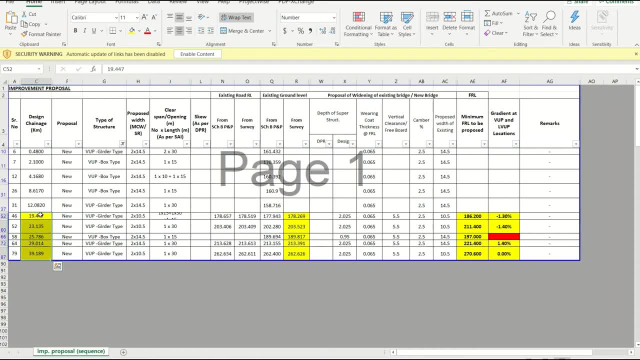 project. see chain edges. we have to mention at what chain is. what type of structure is there? can you see there are two types. one is gutter type structure and a box type structure. in gutter type some depth depth of superstructure will be higher. okay, in box type depth of. 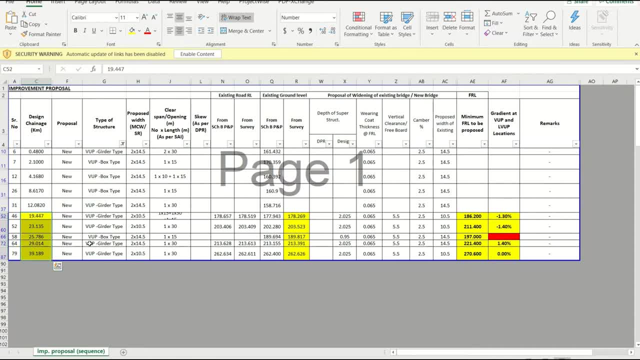 superstructure will be less so. first we have to mention the chain edges and then type of structure- okay, whether it might be gutter type or box type. then proposed width, based on the cross section, what i have shown earlier- and then span arrangement, that that can be decided by. 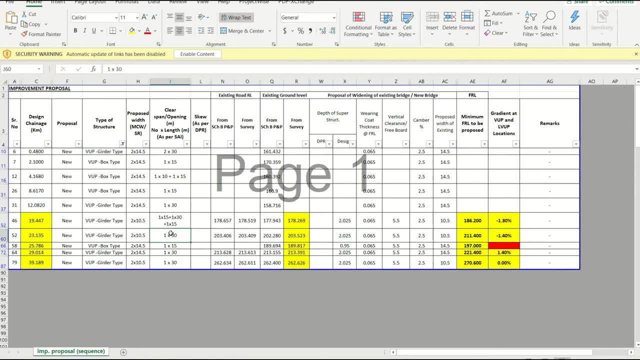 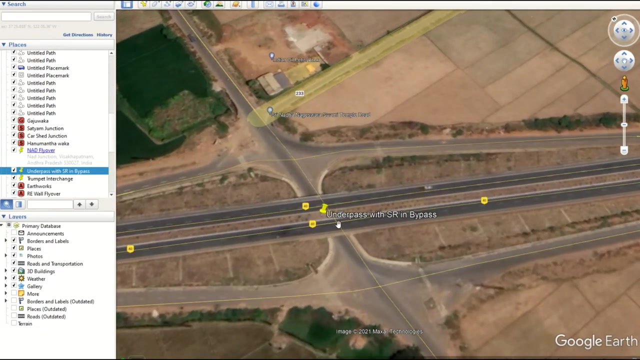 by the structure structure team, okay, and then- and based on the crossroad also you have to decide- then structure team will decide okay, and then after that survey means original level, ogl, ground level at the this chain, edge, particular chain, okay here. crossroad level, here, exactly at the center or whatever may be average you can also take okay, so original ground. 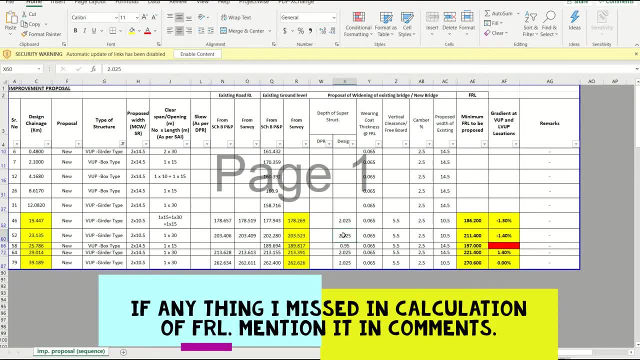 at this look and then depth of superstructure. i told it will vary based on the type of structure- workauda or box- so that you have to mention here then varying coat wearing coat thickness, the standard 65 mm, then vertical clearance. this will be from the code as i uh. 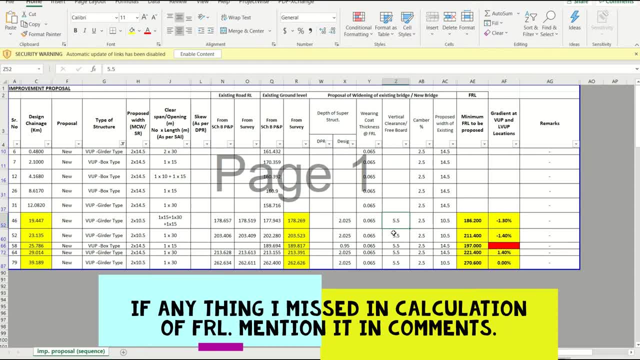 showed in ircsp 84, you have to take a specific clearance. okay, if you add a luvp 3.5 meter, or else vup 5.5 meter. if it is a cup, three meters is enough. okay, so then camber, normal, camber, whatever. 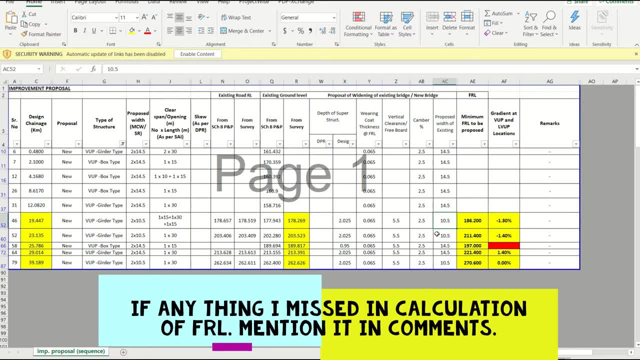 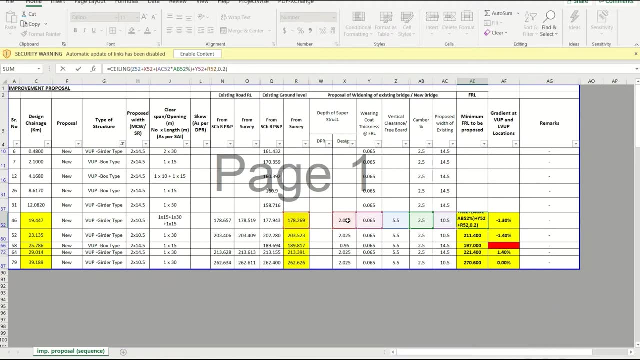 the camber you are providing that you have to mention, then proposed width, mention width of the plane, okay, and structure that then you have to calculate the frl how it has been calculated: existing survey plus 2.025, plus this 0.065 varying code, and then clearance 5.5 and then this 10.5. 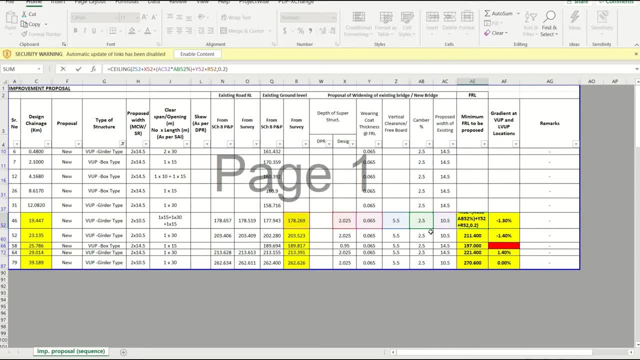 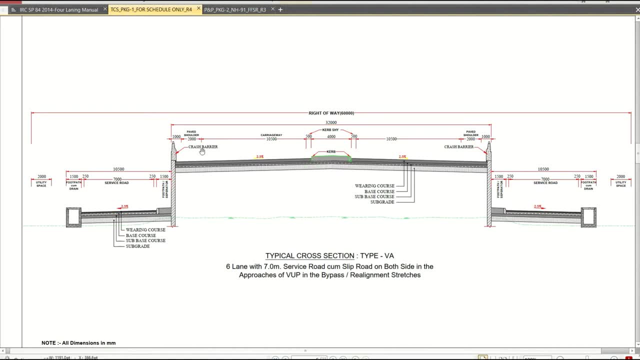 into 2.5 that you have to calculate because a section see ground level and then clearance: 5.5 meter normal deck level, deck deck means a depth of that superstructure will come okay and then varying code of once the frl is calculated means there are various criterias, some sag, correction and overlay. 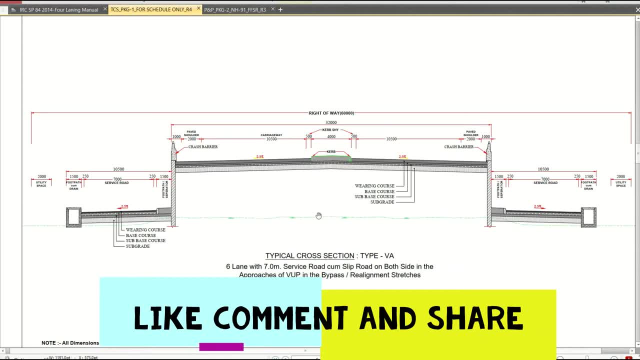 if existing junction is there, how much overlay we are going to provide. so, like that, some few extra criterias you have to consider while deciding the frl, but basic thing is the ground level, plus clearance, plus depth of superstructure, and then varying code and a few thing related to the camber. 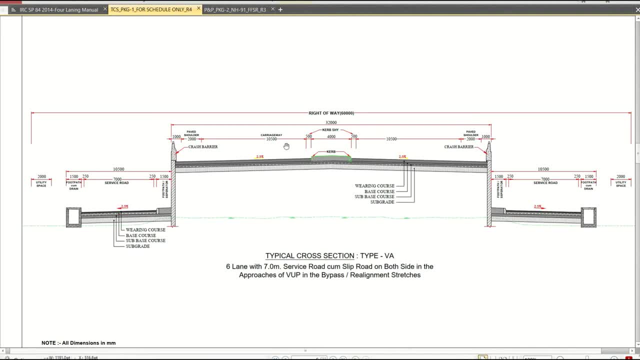 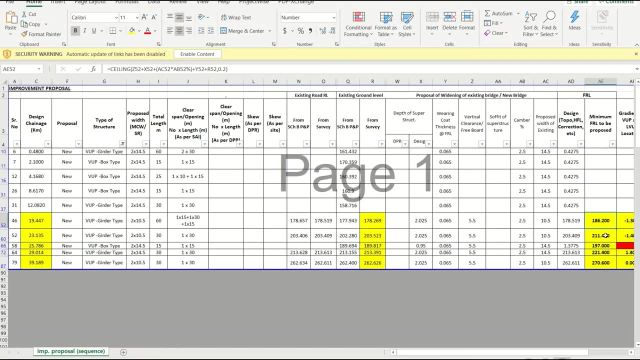 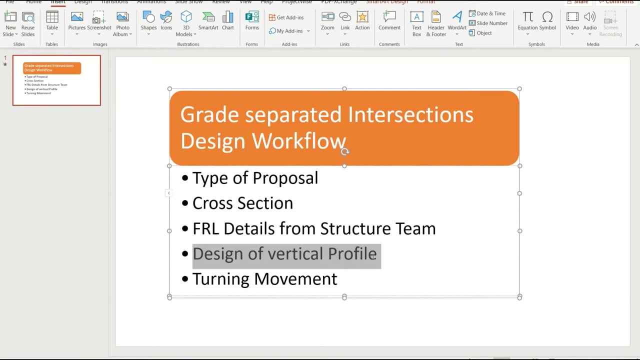 and overlay. so two, three, uh, other criteria based on the all things, you have to decide the frl, what i have shown in the excel sheet. okay, so once you got these values, you have to go to the next step, that is, design of vertical profile. how to do that? we have to do it in a software means either civil. 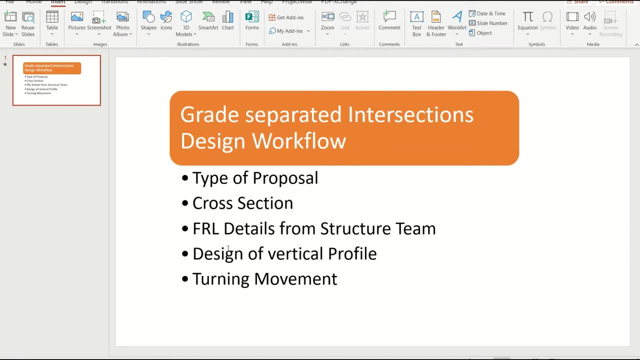 3d or open routes or mx road, but you must be clear about the frl values, the, whatever the structure is coming and at that particular chain is you have to maintain that level. okay, then only it will get satisfied. means design criteria will get satisfied. so 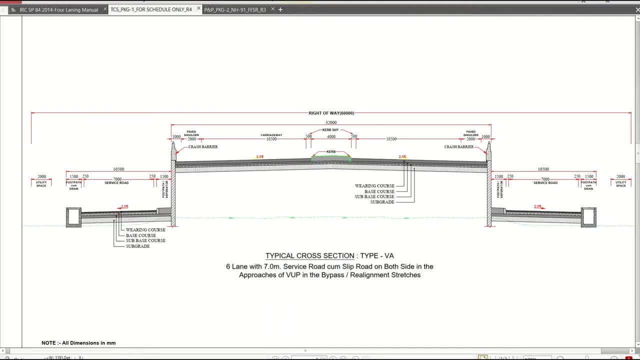 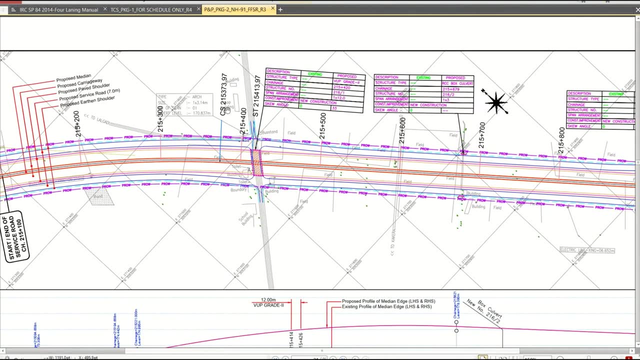 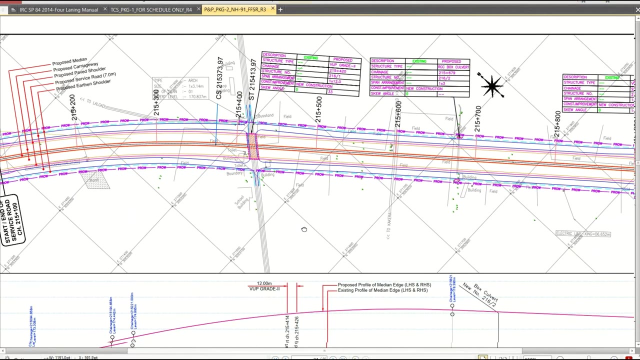 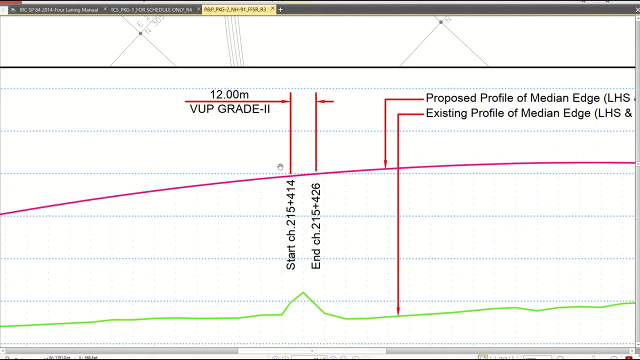 going to the vertical profile. so you have to consider, consider like this: see so here normal road is coming. so and then, at this particular chain edge, can you see this particular chain edge, particular chain edge two, one, five, four, twenty, here this VUP, grade two, and you have 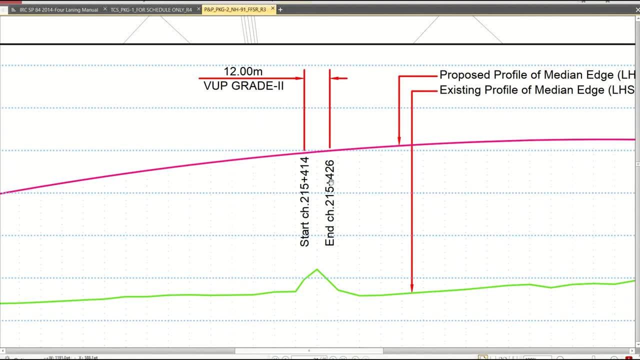 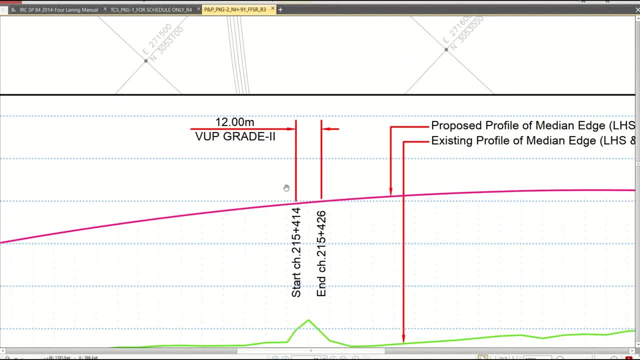 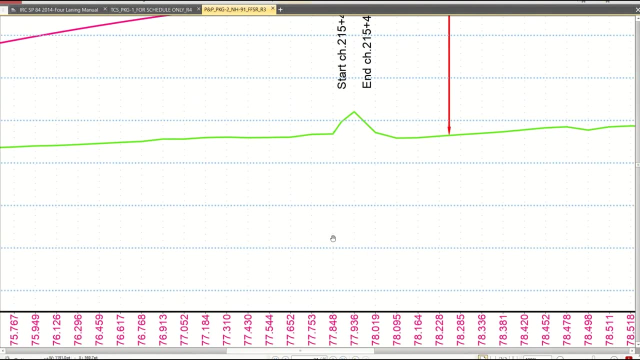 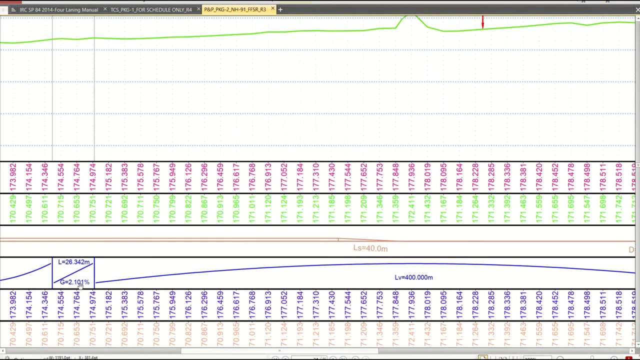 to maintain the referral from that excel sheet using the gradient bearing adjustment and some using so many options in the software. you have to maintain the vertical profile and the. you must satisfy the, the vertical curve length values, also k values, and this vertical curve lengths, k values and gradient gradient should not be more than the desirable. okay, 2.5 percent like. 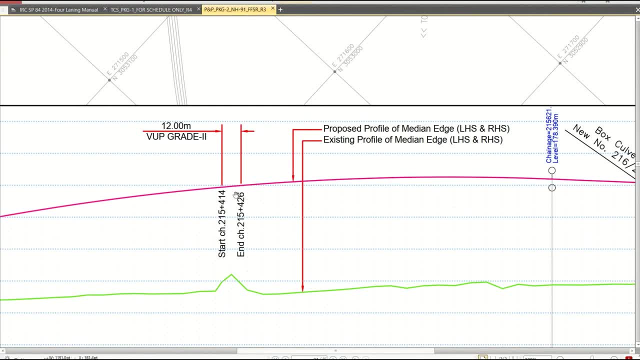 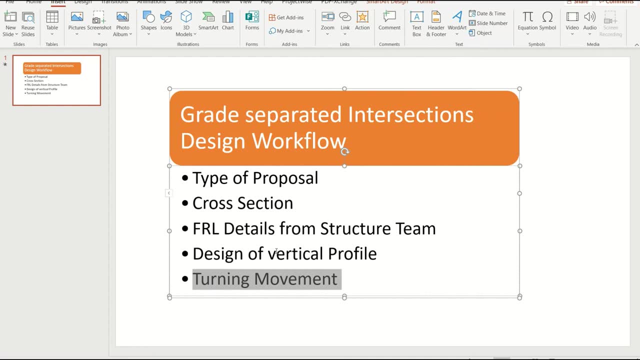 that okay. so you must be aware about this thing. next, turning moment: okay, so you have decided: design the vertical profile and you have run the template and whatever you have done, the line mode also. after that you have to do some proper turning moment options. then only proper moment should be available. so 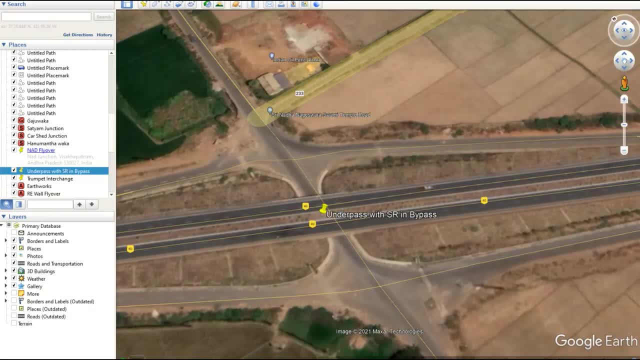 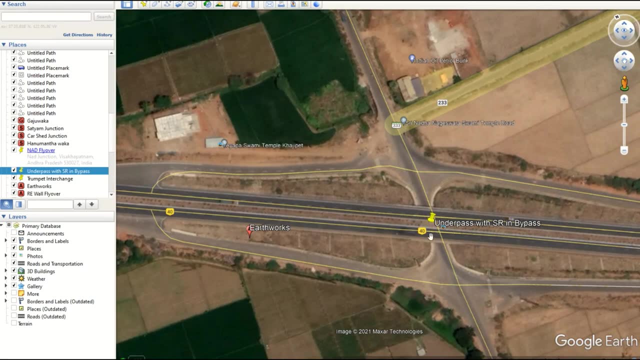 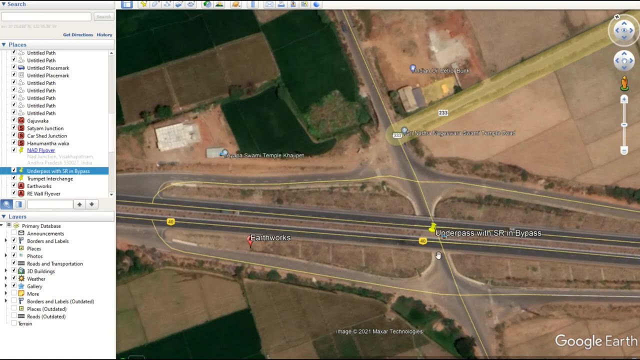 let's have a look. the turning moment. okay, see here itself you can observe. okay, so there must be a proper moment for the trucks. okay, so trucks should be moved easily and there should not be any jam. okay, so for that purpose you have to use auto turn or something like that. so you have to do some.